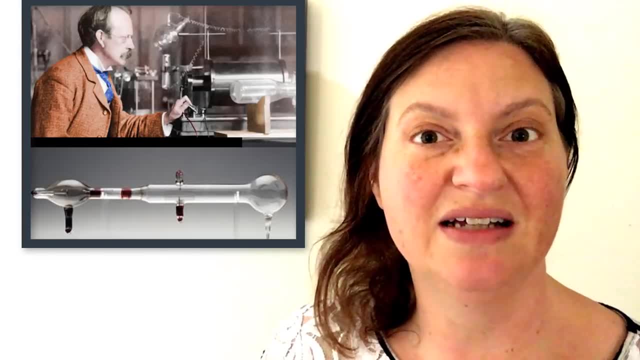 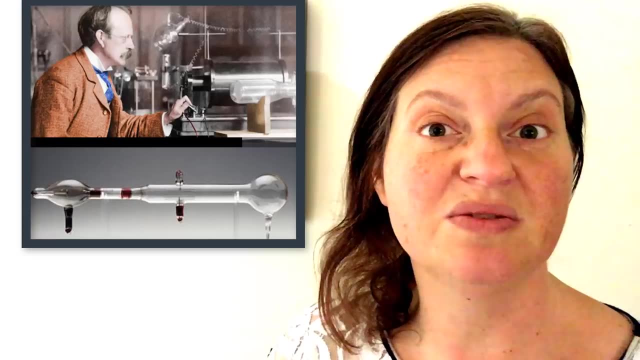 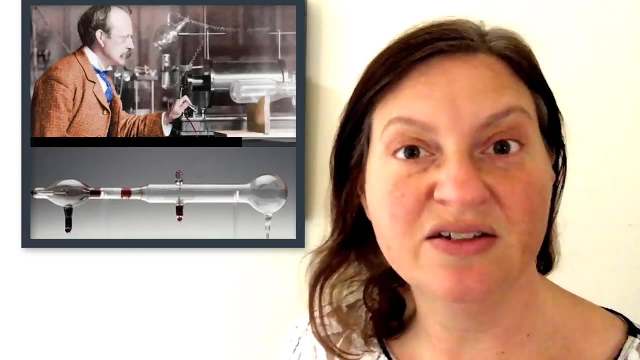 A man named JJ Thompson discovered the electron in 1897, and there are tons of videos about it, but most of them ignore what Thompson himself said was the motivating factor: A debate about how cathode rays move. Want to know not only how, but why electrons were discovered. Let's go. 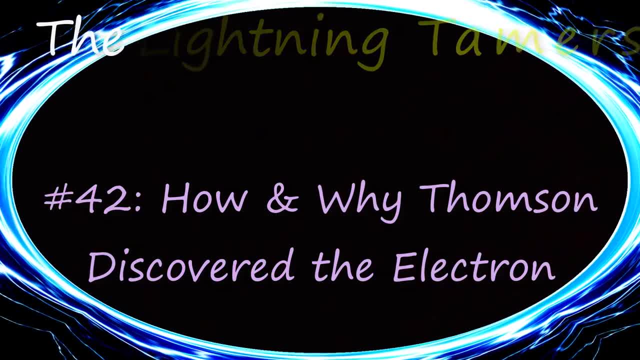 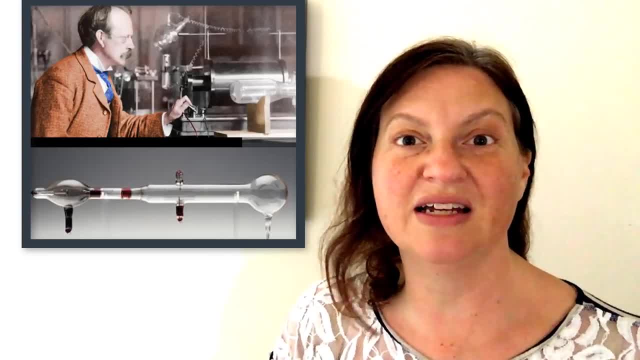 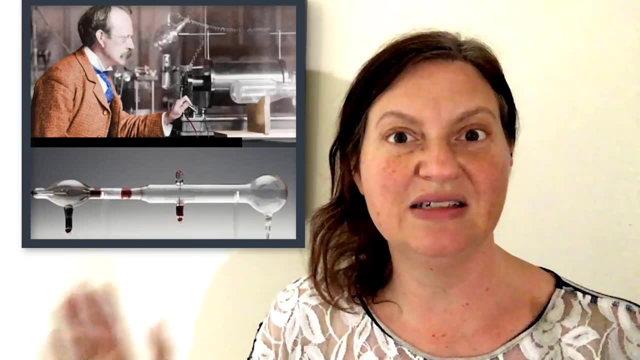 Electricity, electricity. First a little background about Joseph John Thompson: JJ on publications to friends and even to his own son. Thompson was born in Lancashire, England, to a middle-class bookseller. When Thompson was 14, he signed up to be an apprentice to a locomotive engineer. 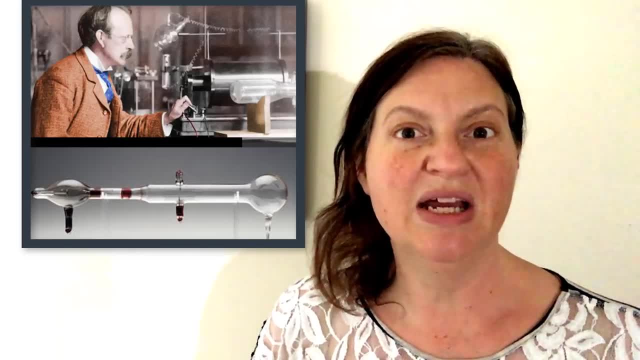 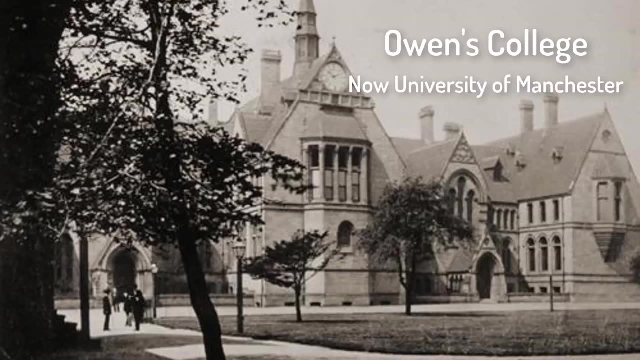 However, they had a long waiting list and to fill the time he applied to and was accepted as a freshman at Owens College. Thompson later recalled that quote. the authorities at Owens College thought my admission was such a scandal. I expect they feared that students would soon be coming in strollers. 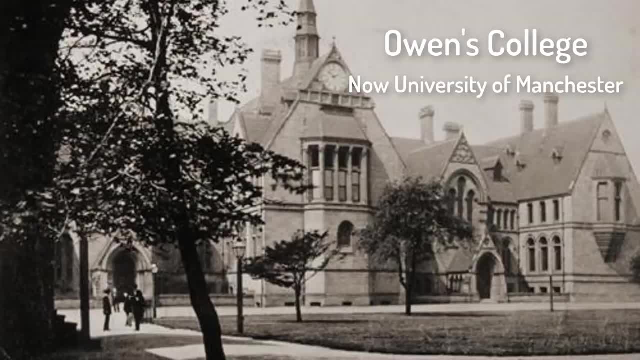 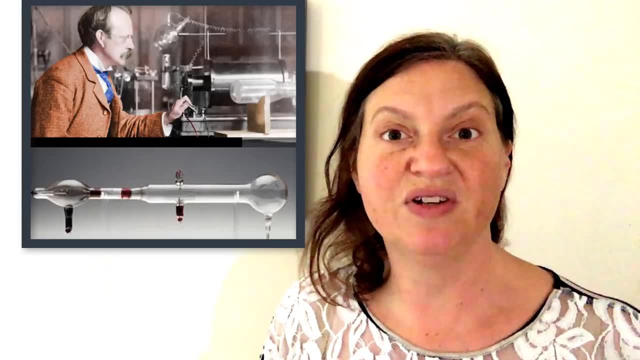 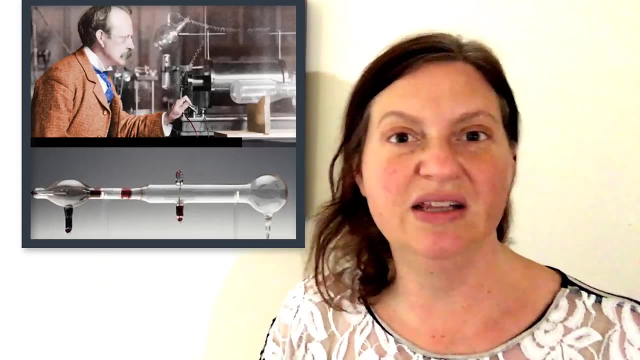 that they passed regulations raising the minimum age for admission so that such a catastrophe should not happen again. While in school, Thompson's father died and they didn't have enough money for him to get the apprenticeship. Instead he relied on scholarships at university, ironically leading him to greater fame In 1884, at the tender age. 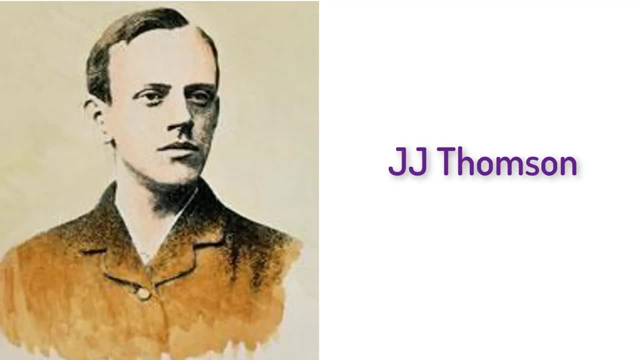 of 20, he became a professor at the University of New York. He was a professor at the University of New York In 1928, Thompson applied to be the head of the Cavendish Research Institute. He mostly applied as a lark and was surprised as anyone to get the position He said, quote: I feel like a. 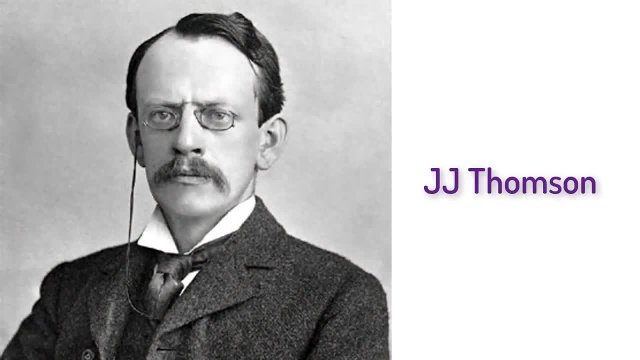 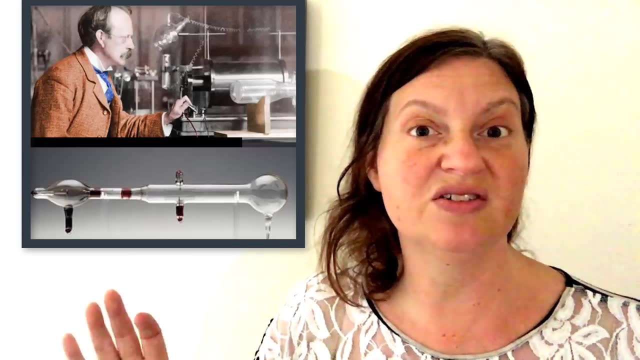 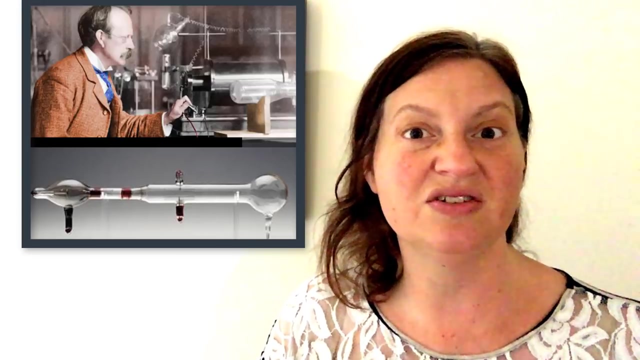 fisherman who has cast a line in an unlikely spot and hooked a fish much too heavy for him to land. Suddenly, Thompson had a lot of resources, stability and ability to research whatever he wanted. He ended up having an uncanny ability to find new material to research, In fact, a full 8. 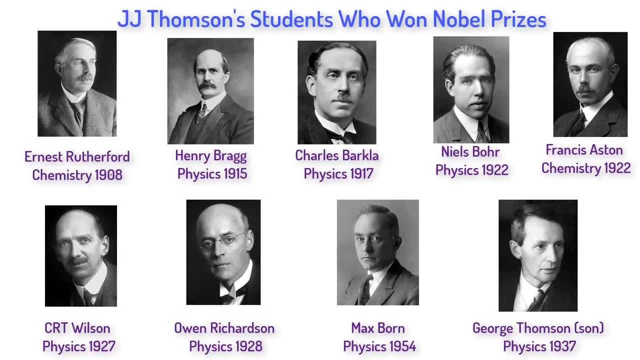 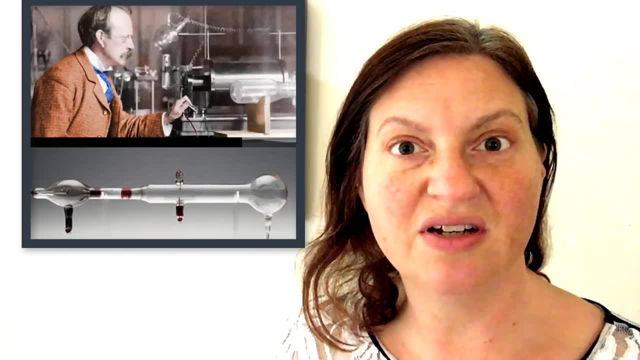 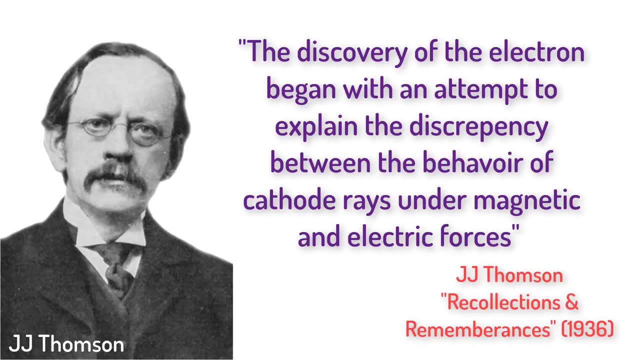 of his research assistants and his son eventually earned Nobel Prizes, But, of course, like Thompson's own Nobel Prize, that was in the future. Why did JJ Thompson discover the electron in 1897?? Well, according to his autobiography quote, the discovery of the electron began with an attempt to 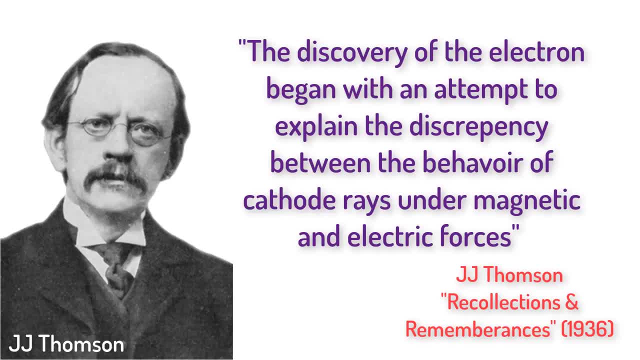 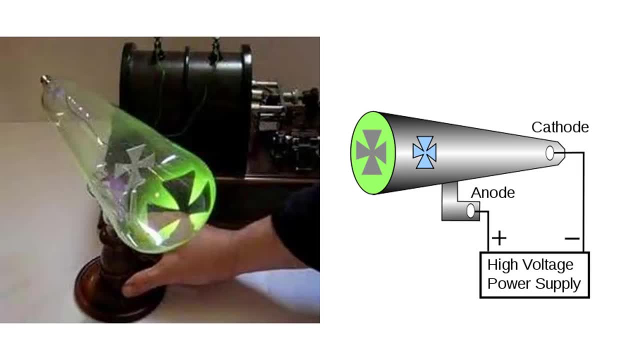 explain the discrepancy between the behavior of cathode rays under magnetic and electric forces. What did he mean by that? Well, a cathode ray or a ray in a vacuum tube that emanates from the negative electrode can be easily moved with a magnet. This fact gave a charismatic English chemist named 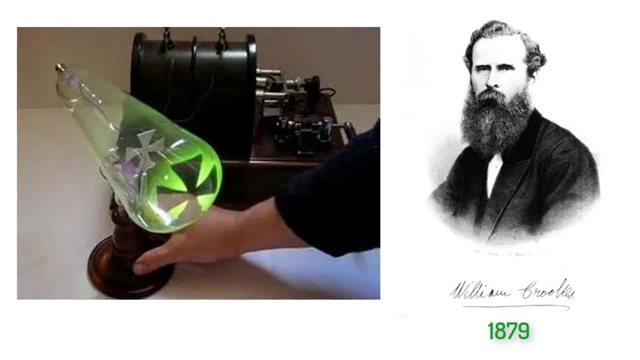 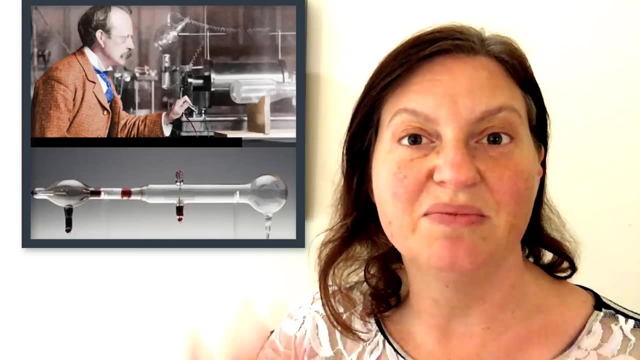 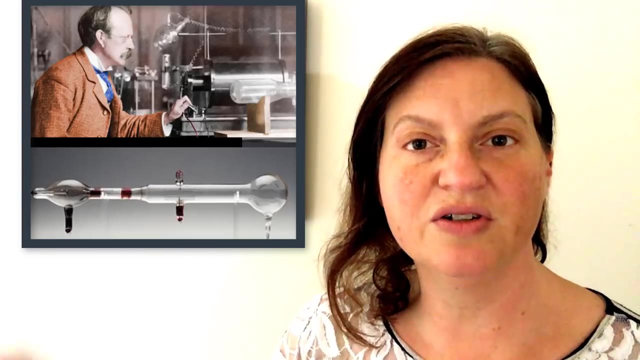 William Crookes the crazy idea that the cathode ray was made of charged particles in 1879. However, five years later a young German scientist named Heinrich Hertz found that he could not get the beam to move with parallel plates or with an electric field. Hertz decided that Crookes was. 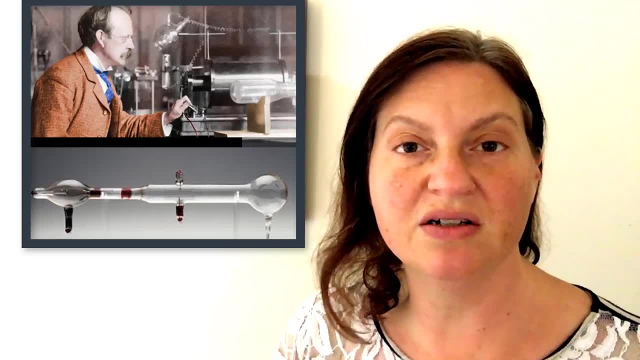 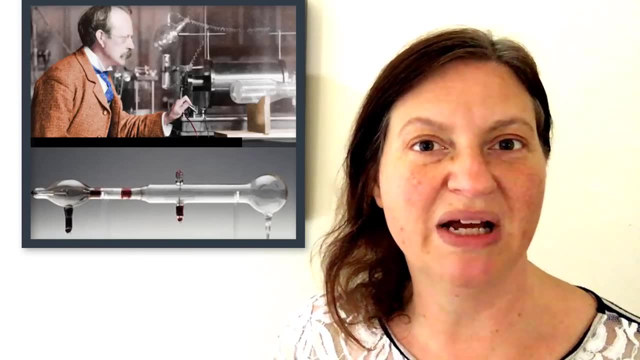 wrong. If the cathode ray was a beam of charged particles, then it should be attracted to a positive plate, and if it was a beam of charged particles, then it should be attracted to a positive plate and repelled from the negative plate. And Hertz decided it was some kind of new electromagnetic. 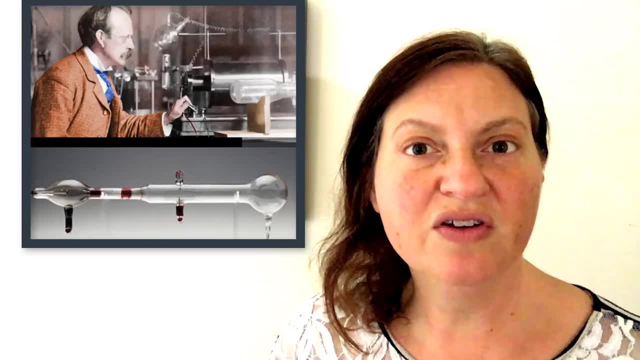 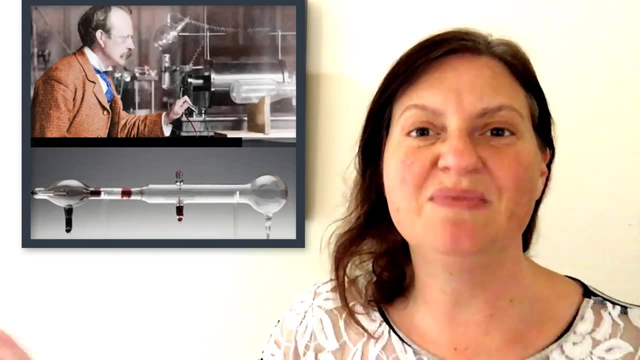 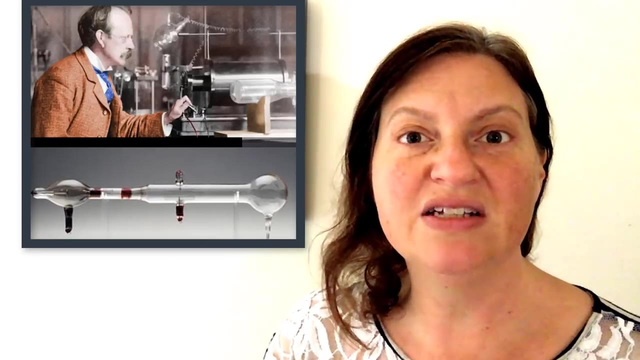 wave like a new kind of ultraviolet light. Further in 1892, Hertz accidentally discovered the cathode rays could tunnel through thin pieces of metal, which seemed like further proof that Crookes was so very wrong. Then, in December of 1895, a French physicist named Jean Perrin 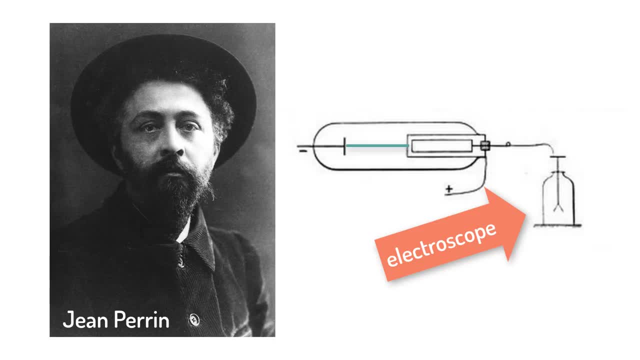 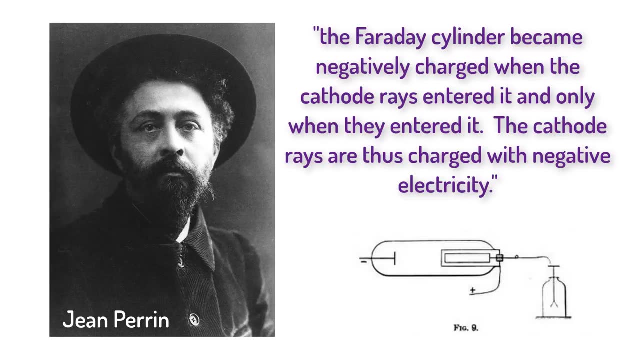 used a magnet to direct a cathode ray into and out of an electroscope called a Faraday cylinder and measured its charge. Perrin wrote, quote: the Faraday cylinder became negatively charged when the cathode rays entered it, and only when they entered it. The cathode rays are thus 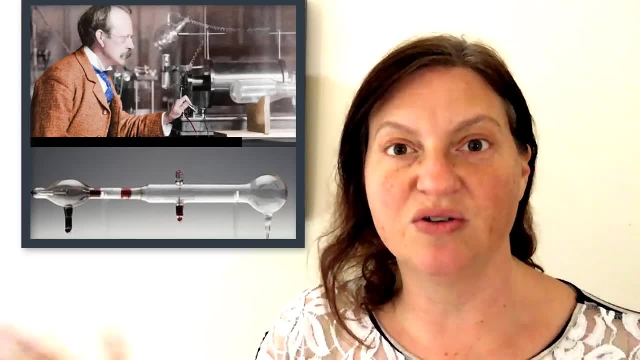 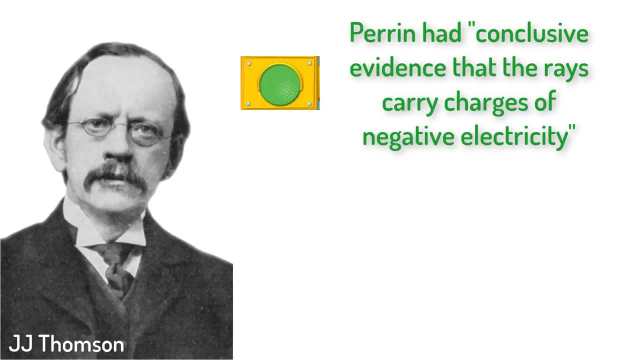 charged with negative electricity. This is why JJ Thompson was so confused. He felt that Perrin had quote conclusive evidence that the rays carried a charge of negative electricity, except that quote Hertz had found that when they were exposed to an electric force they were not deflected at. 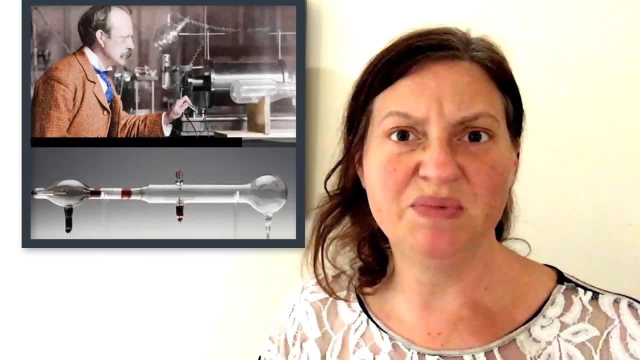 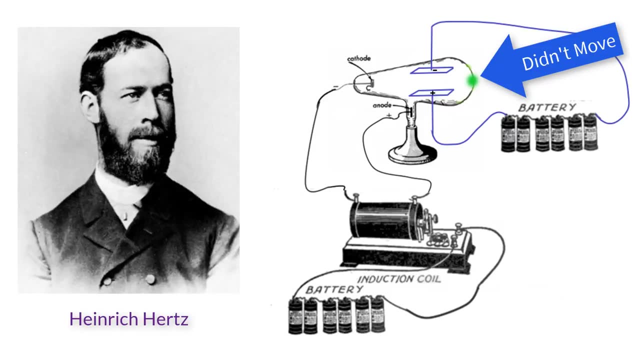 all. So what was going on? Thompson wondered if there might have been something wrong with Hertz's experiment with the two plates. Thompson knew that the cathode ray tubes that they had only work if there's a little bit of air in the tube, and Thompson wondered if the air affected. 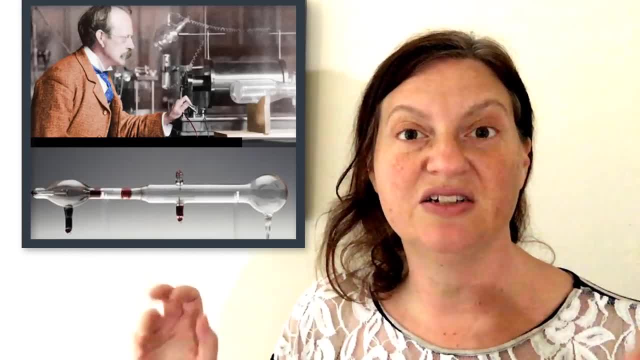 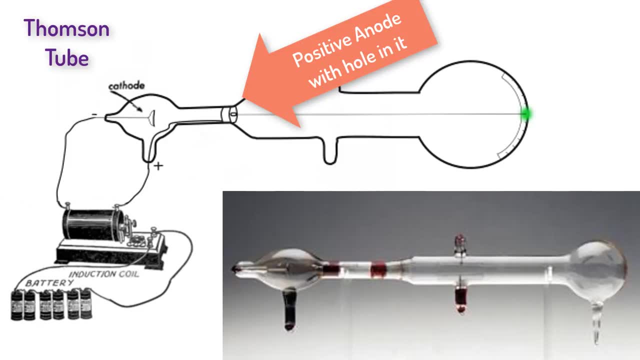 the results. Through trial and error, Thompson found he could get a stronger beam by shooting it through a positive anode with a hole in it. With this system he could evacuate the tube to a much higher degree And if the vacuum was good enough, the cathode ray was moved by electrically. 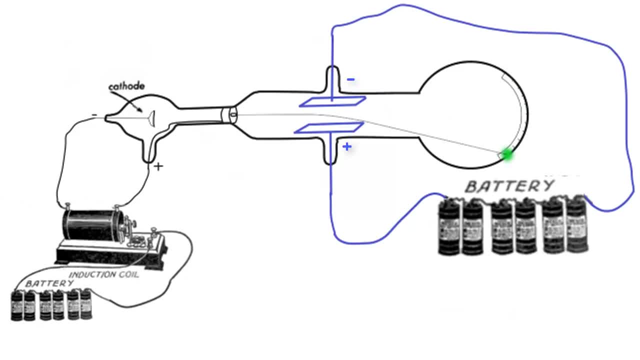 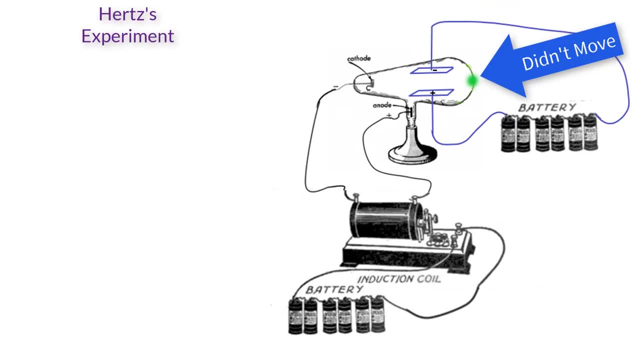 charged plate, just as negatively electrified particles would be. If you're wondering why the little bit of air affected it, it's because the air became ionized in the higher electric field and became conductive. The conductive air then acted like a Faraday cage, shielding the beam from 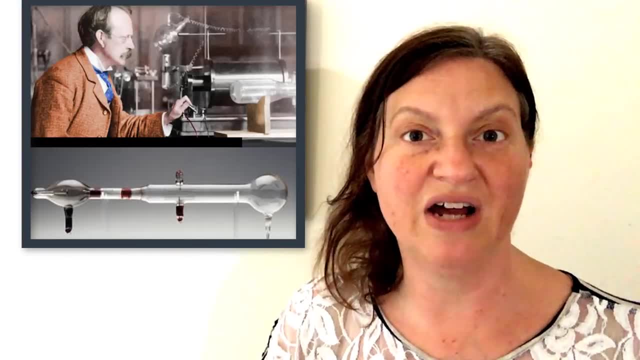 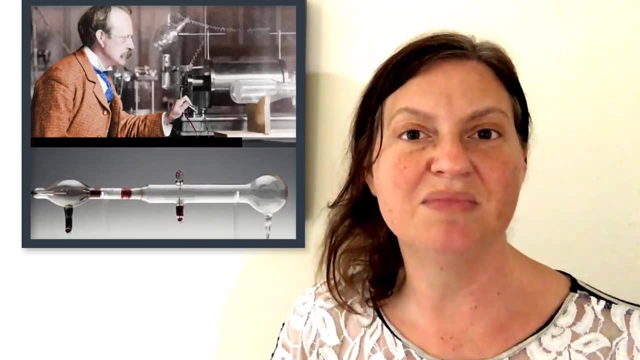 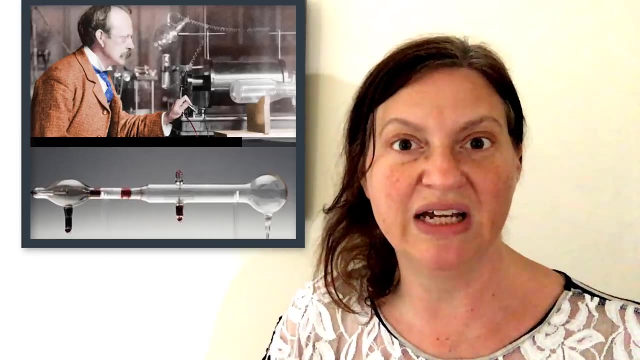 the electric field. As stated before, Heinrich Hertz also found that the cathode ray could move through thin metals. How could a particle do that? Well, Thompson thought maybe particles could do that if they're moving really, really fast. But how to find how fast the cathode beam was moving? He used the fact that he could. 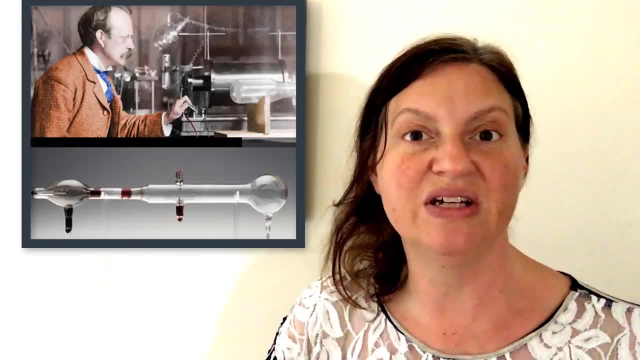 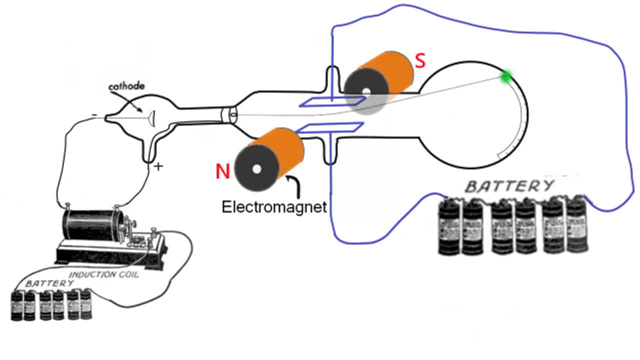 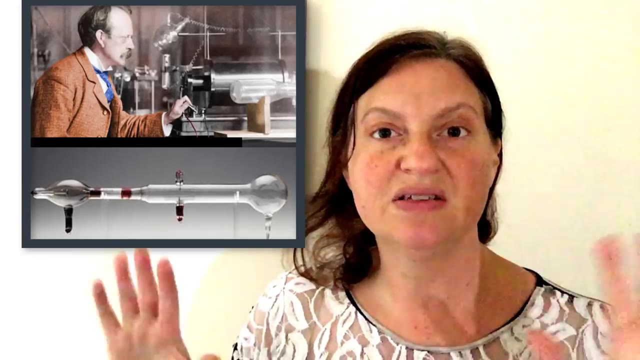 move it both with an electric field and a magnetic field to make an electromagnetic gauntlet. First Thompson put a magnet near the ray to deflect the ray one way, and then he added charge to the plates so that the forces were balanced and the ray went in a straight line. Thompson knew that the force 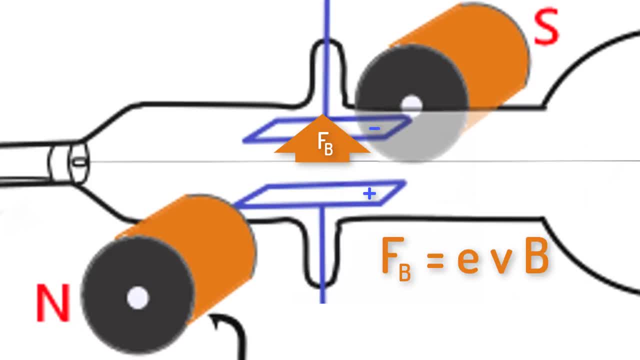 from the magnet depended on the charge of the particle, its speed and the magnetic field. He also knew that the electric force from the plates only depended on the charge of the particle and the electric field. Since these forces were balanced, Thompson could determine the speed of the particle from the ratio. 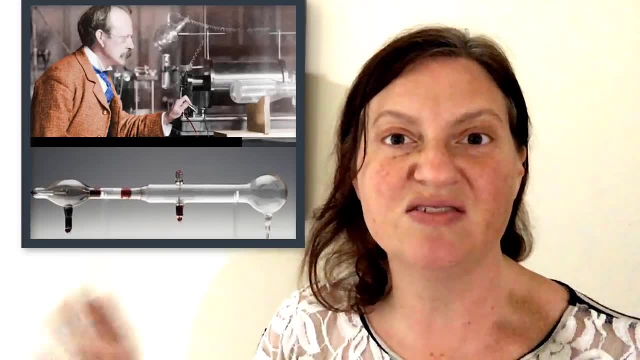 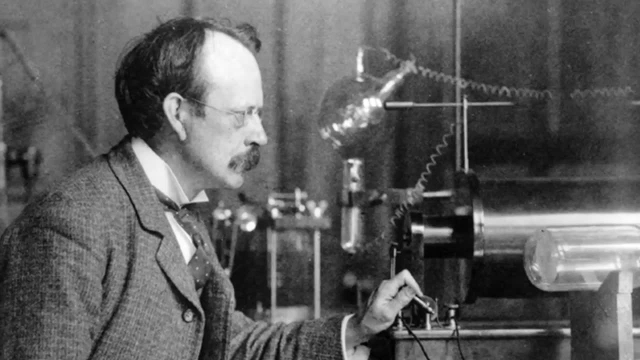 of the two fields, Thompson found speeds up to 60,000 miles per hour, or up to a third of the speed of light. Thompson recalled quote: in all cases where the cathode rays are produced, their velocity is much greater than the velocity of any other moving body which we have. 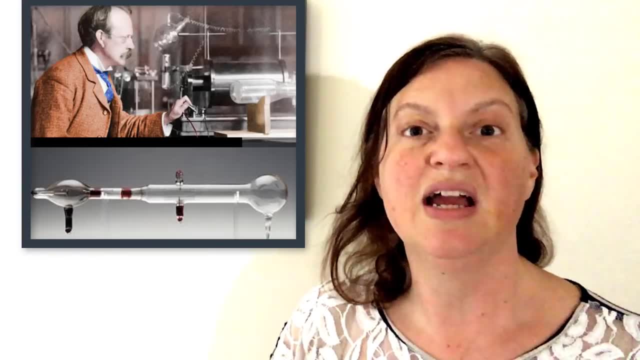 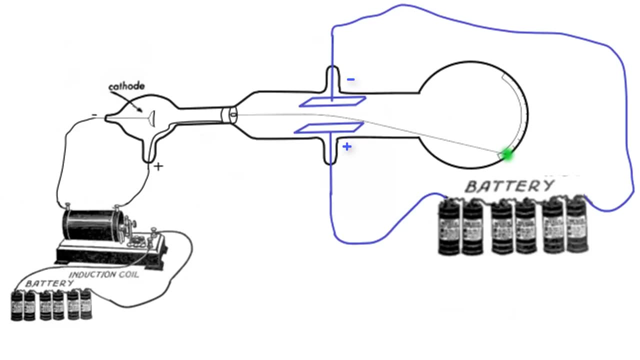 Thompson then did something even more ingenious: He removed the magnetic field. Now he had a beam of particles moving at a known speed, with a single force on them, They would fall, as Thompson said, quote, like a bullet projected horizontally with velocity v. 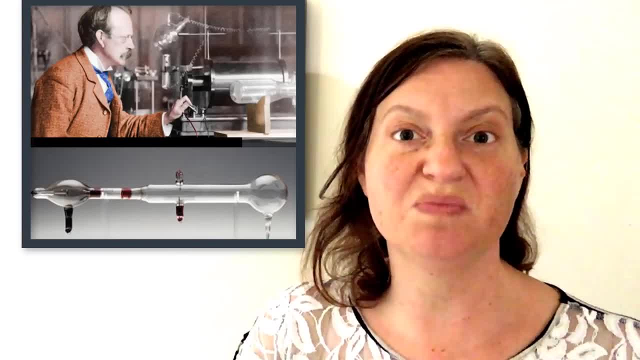 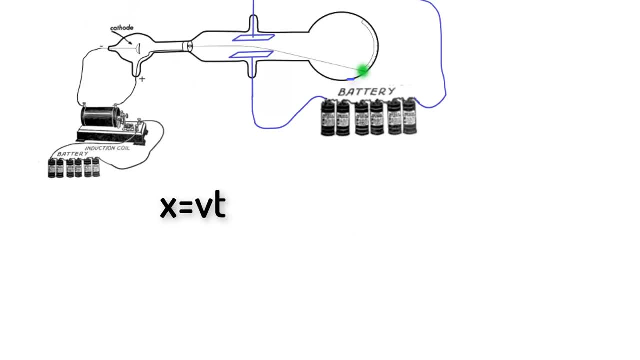 Note that the gravitational force is much, much smaller than the electric force on such light objects and therefore can be ignored. By measuring the distance the cathode ray went, he could determine the time they were in the tube and by the distance they fell, Thompson could determine. 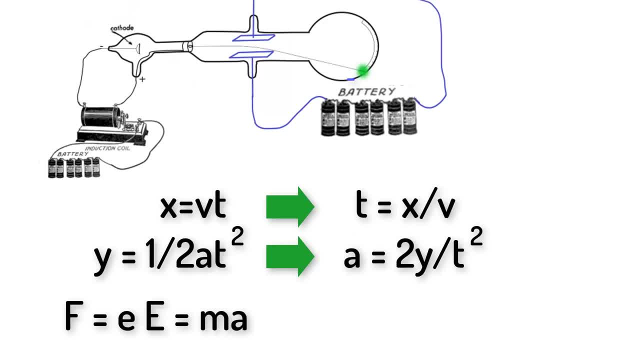 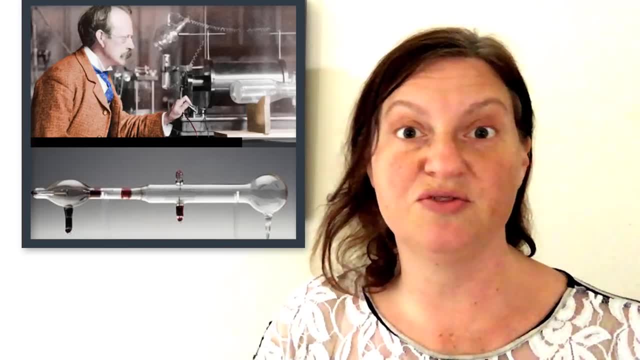 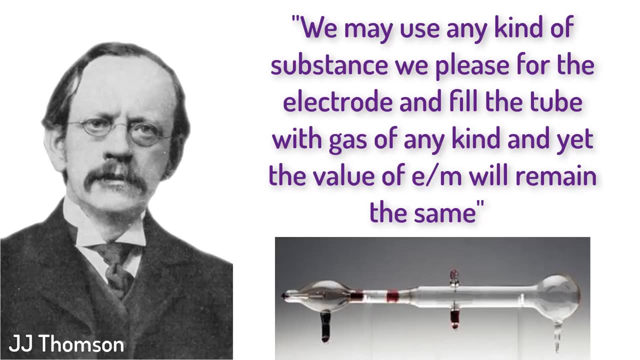 their acceleration. Using f equals ma. Thompson determined the ratio of the charge on the particle to the mass, or e over m. He found some very interesting results. First, no matter what he changed about the experiment, the value of e over m remained constant. Quote: we may use any kind of. 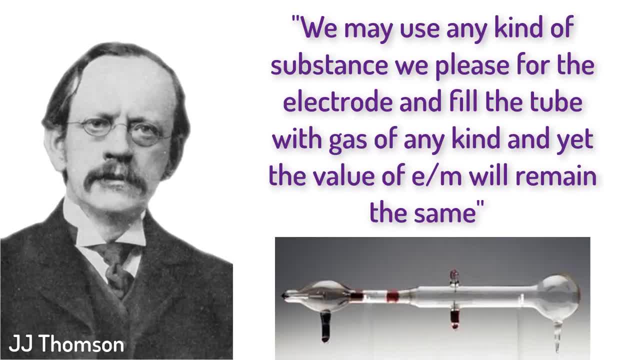 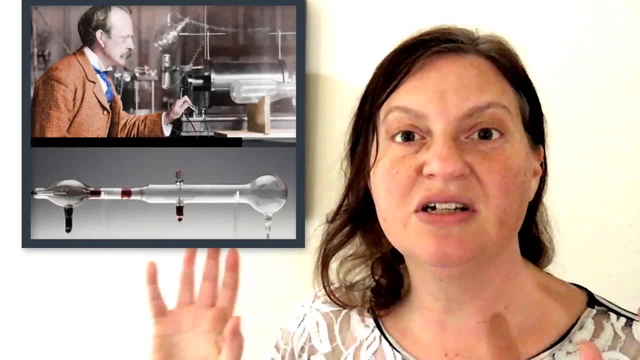 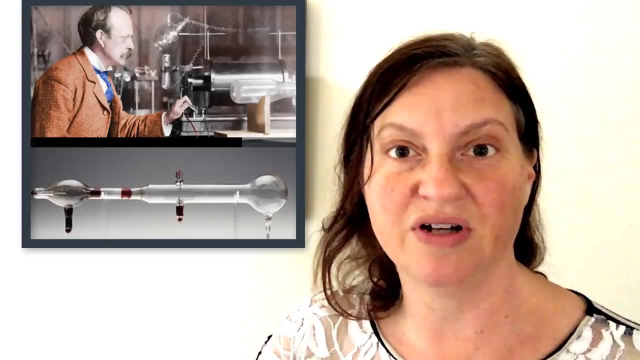 substance. we please for the electrodes and fill the tube with gas of any kind, and yet the value of e over m will remain the same. This was revolutionary. Thompson concluded that everything was filled with these tiny little things that he called corpsicles but we now call electrons, and 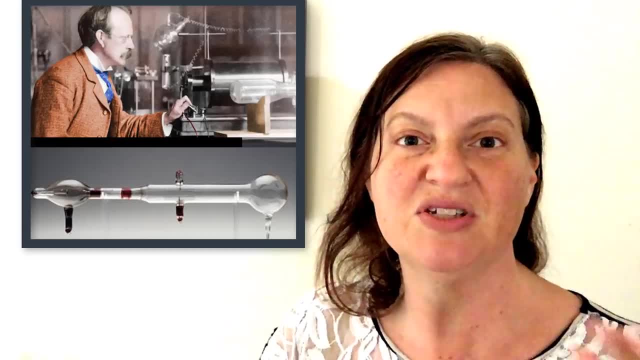 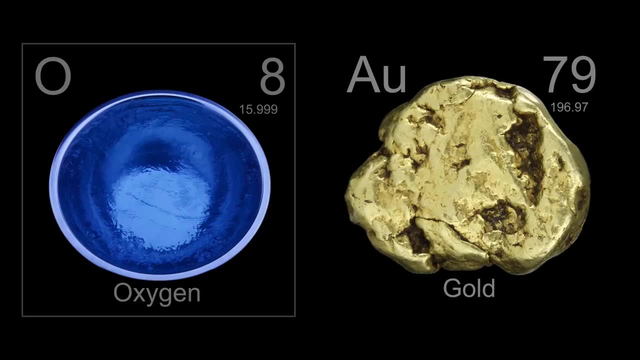 that the corpsicles in one item are exactly the same as the corpsicles in another. So, for example, an oxygen molecule contains the same kind of electrons as a piece of gold. Atoms are the building blocks of matter, but inside the atoms there are these tiny electrons. 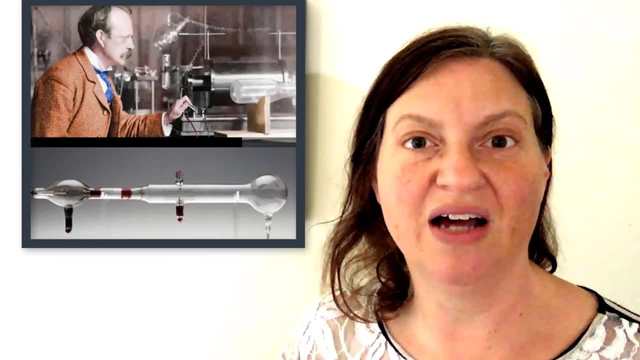 that are the same size as a piece of gold. The atoms are the building blocks of matter, but inside the atoms there are these tiny electrons that are the same size as a piece of gold. Same for everything. The other crazy result he found was the value of e over m was enormous. 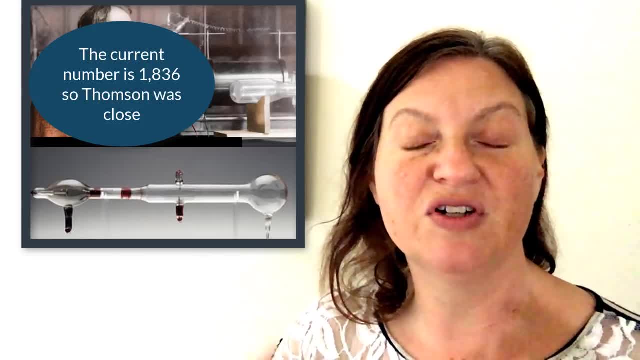 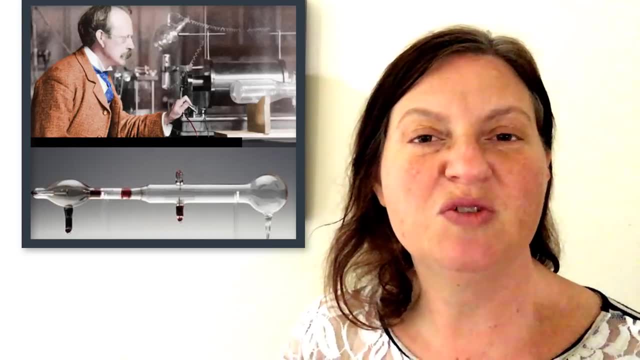 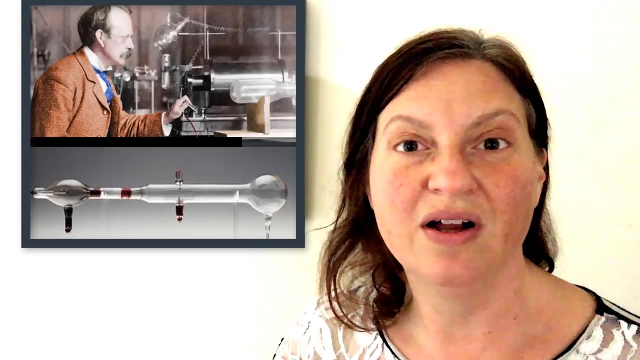 about 1700 times bigger than that for a charged hydrogen atom, which had the biggest value of e over m for anything they had found before, which meant that either these corpsicles were very, very highly charged or they were tiny. A student of Thompson's named CTR Wilson had experimented. 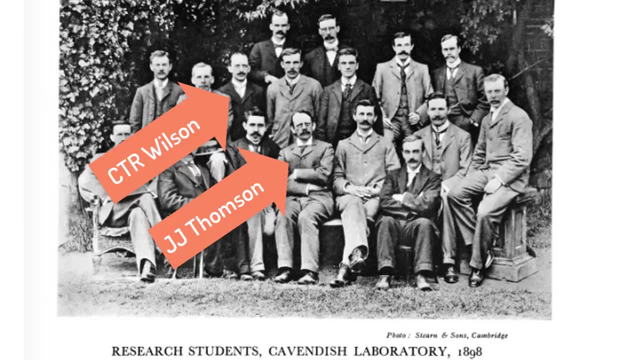 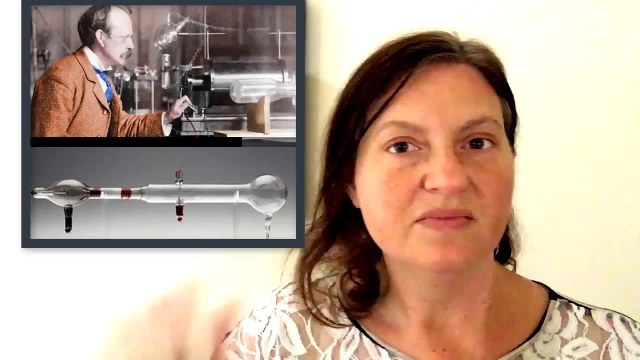 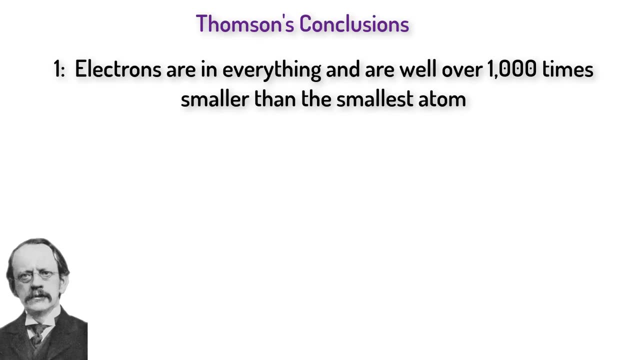 with slowly falling water droplets and found that the charge on the corpsicles were, to the accuracy of the experiment, the same as the charge on a charged hydrogen atom. Thompson therefore came to some really interesting conclusions. One, electrons are in everything and are well over a thousand. 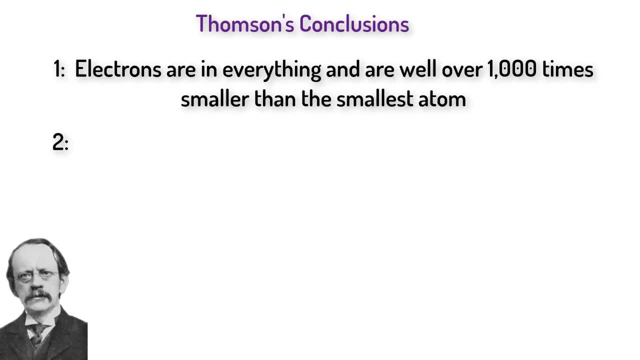 times smaller than even the smallest atom. Two: Benjamin Franklin thought positive objects had too much electrical fire and negative had too little. Really, positive objects have fire, have too few electrons and negative have too many, Oops. three, although, since Franklin, 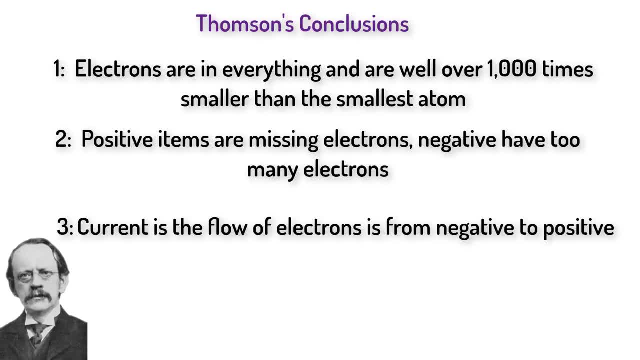 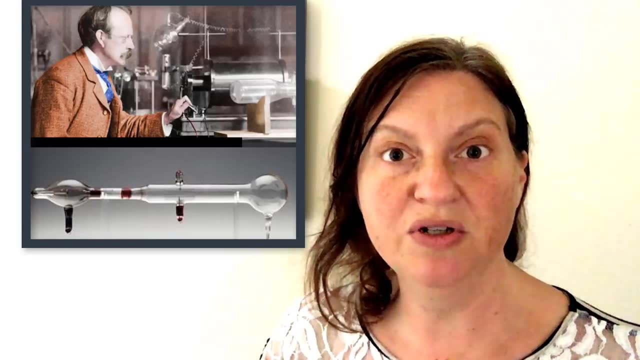 people thought current flow from positive to negative. really, the electrons are flowing the other way. When a person talks about the current that flows from positive to negative, they're talking about something that is not real. True electrical current flows from negative to positive and that's the way the electrons move. 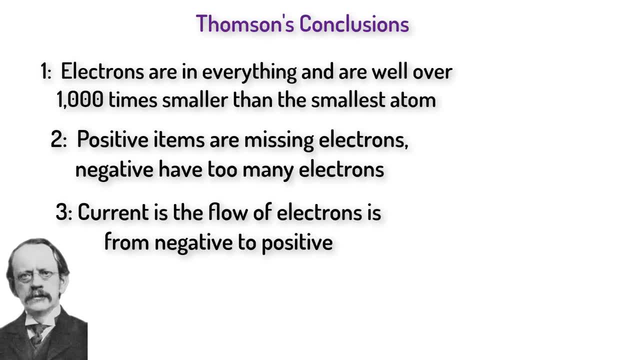 However, by the time people believed JJ Thompson, it was too late to change our electronics, So people just decided to stick with. quote: conventional current going the wrong way. Sorry four, since electrons are tiny and in everything but most things, have a neutral charge. 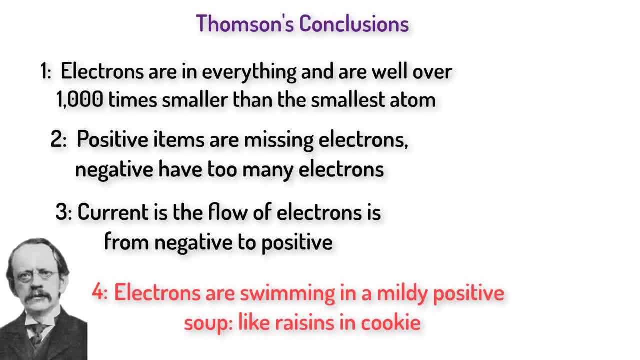 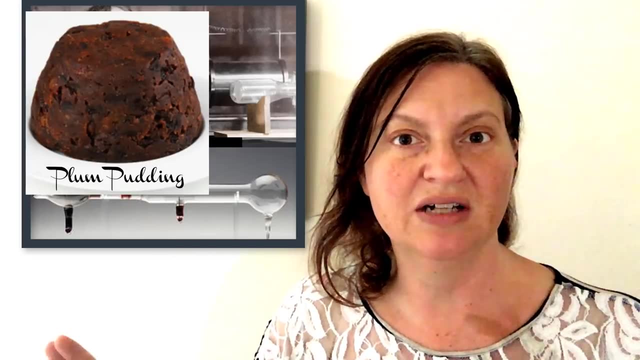 and because solid objects are solid, the electrons must be swimming in a sea or soup of mildly positive material, like raisins in a raisin cookie. The first three conclusions are still considered correct over a hundred years later. The fourth theory is called the plum pudding model.